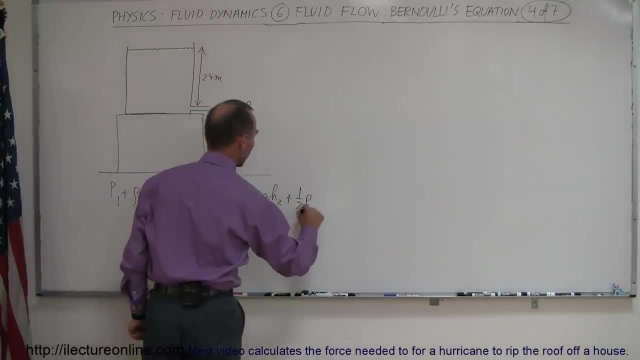 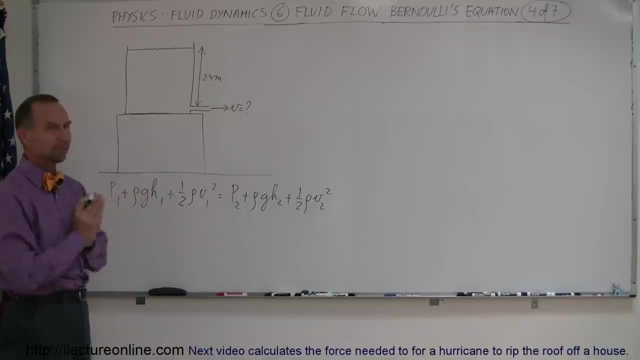 call it h plus one-half rho, v2 squared. Okay, now that we have the equation, we have to identify point 1 and point 2.. Let's call this here point 1, and let's call this right here point 2.. So what is the pressure? 1,? 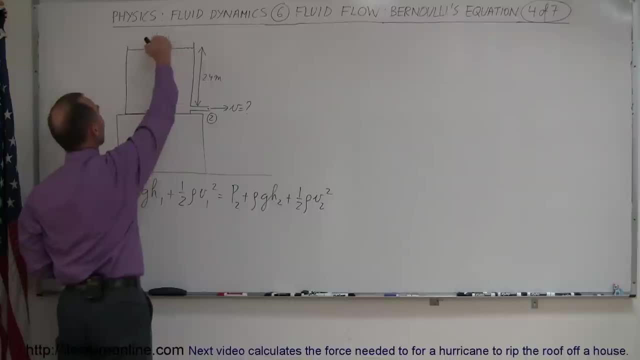 what is the pressure at 2?? Well, it's open to the atmosphere. so at point 1, that would be atmospheric pressure, so P atmosphere. Now at point 2,, right at the opening where the water comes out, and assuming that this is water, h2o, then the pressure there would also be at the 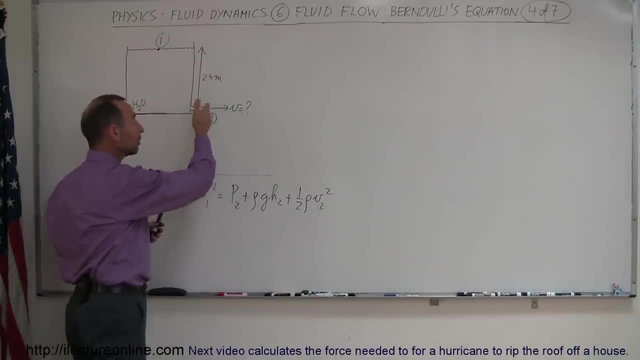 atmospheric pressure because it's exposed to the atmosphere. so at that moment pressure would be atmospheric pressure. so we can say this is equal to P atmosphere. All right now, what's the velocity of the water at point 1?? Well, since this is a very small opening and this is a very big, 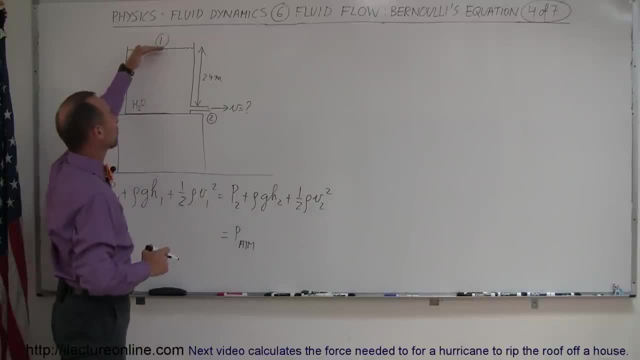 tank with a lot of water. the water would drop extremely slowly here compared to the water coming out over here. So we can say that for all intents and purposes, the velocity of 1 would be zero. That means that this term would become zero. so 1 half rho times zero squared, so this whole term. 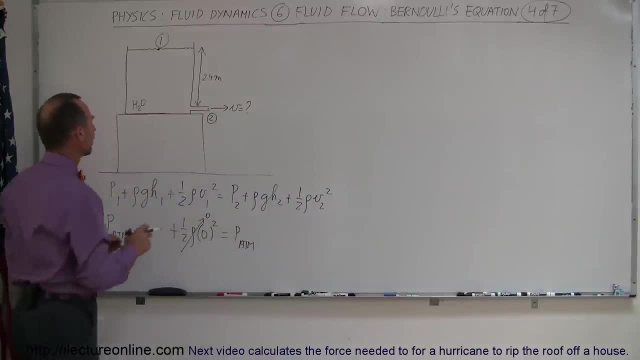 goes to zero. Now, height-wise we can say that if we call this our reference height, then the height of 1 would be 2.4 meters above height of 2, and of course height of 2 then equals zero. 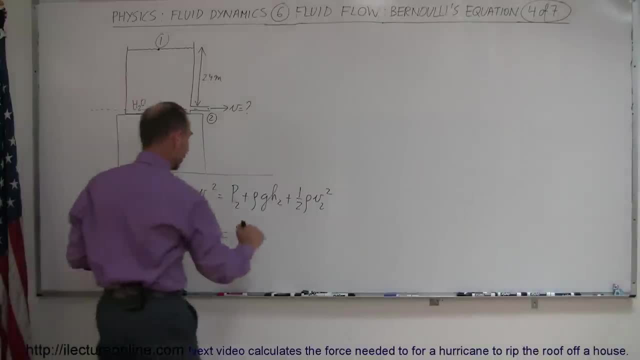 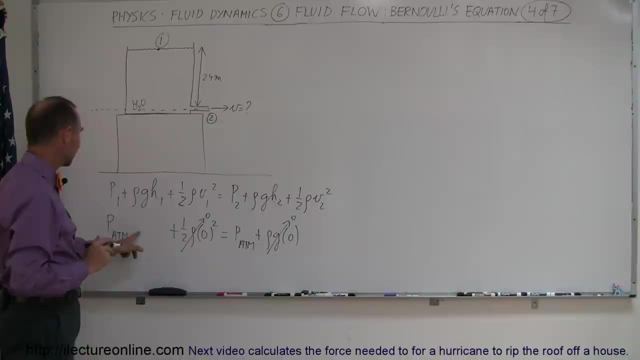 because that's our reference height. We can pick it anywhere we like. so that means that this becomes plus rho g times zero, and so that term would go to zero. Then all we have left is right here is rho gh1,. so plus rho gh1, and over here we have plus. 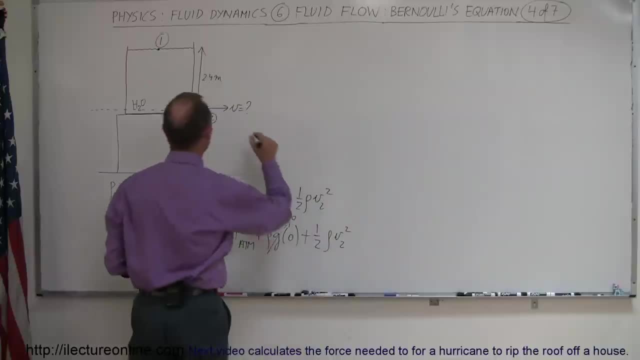 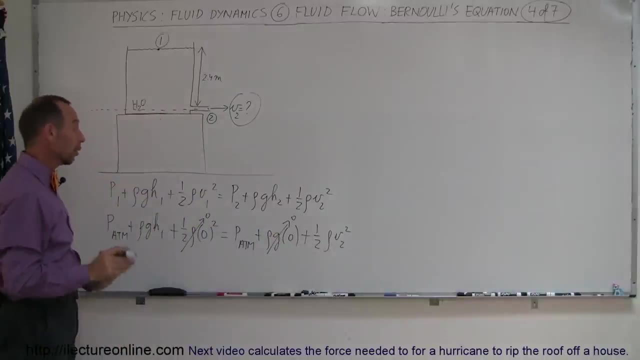 1 half rho, v2 squared and, by the way, this is v2.. That is what we're looking for, looking for v2.. Also, since the two places here- point 1 and point 2, are open to the atmosphere, 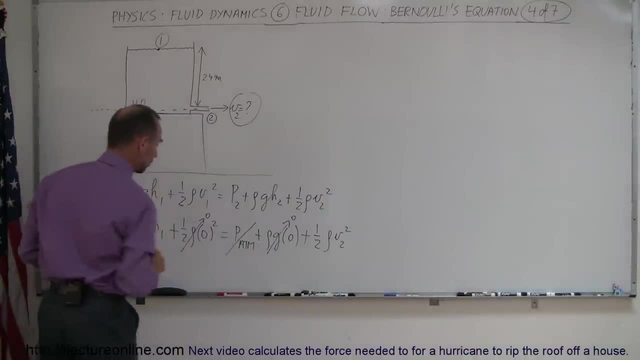 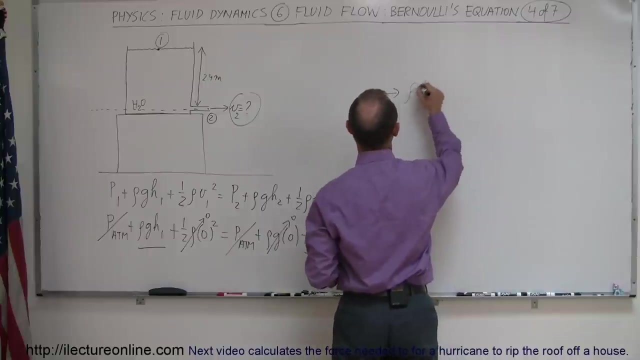 they're both atmospheric pressure, so we can go ahead and cancel atmospheric pressure on both sides of the equation. So we have this term on the left side and this term on the right side. So all that big complicated Bernoulli's equation simplifies to the following: We have rho, gh1. 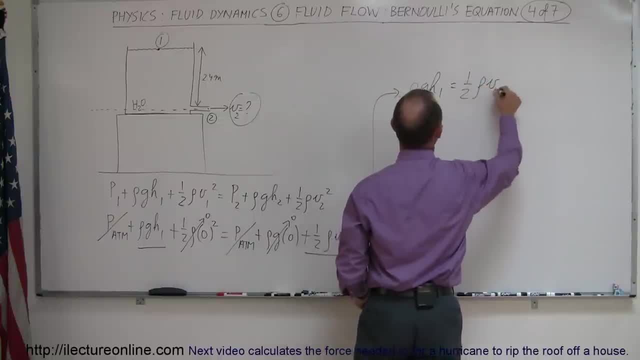 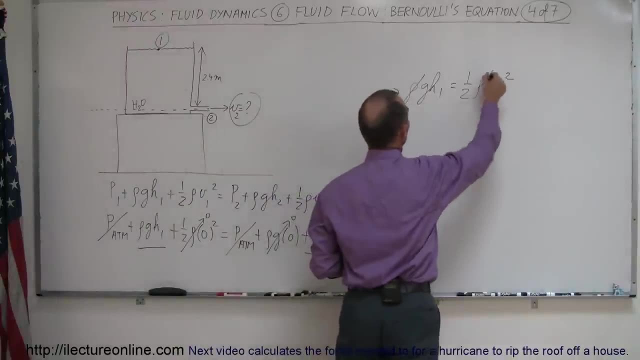 equals 1 half rho, v2 squared. Now you look at that and you realize that on both sides of the equation we have a rho, so that cancels out. This cancels out. with that, Multiplying both sides by 2, we get 2: gh1 equals v2 squared. 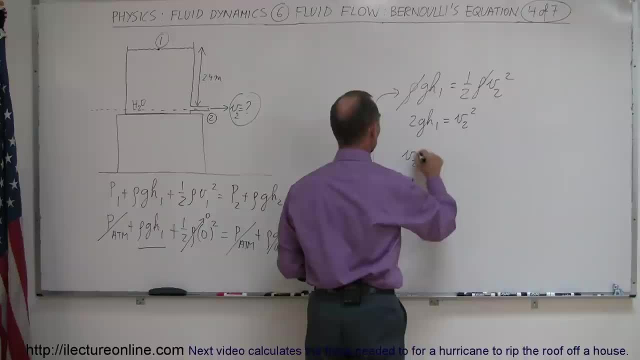 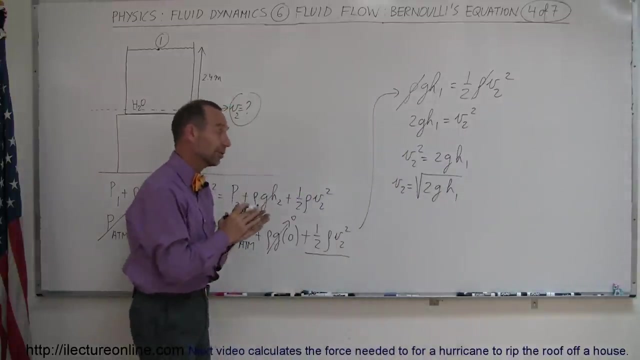 Now I can go ahead and turn the equation around. so we have: v2 squared is equal to 2 gh1, and then if I take the square root of both sides, I can say that v2 is equal to the square root of 2 gh1.. Now that should be an interesting and familiar equation to you. The reason is: 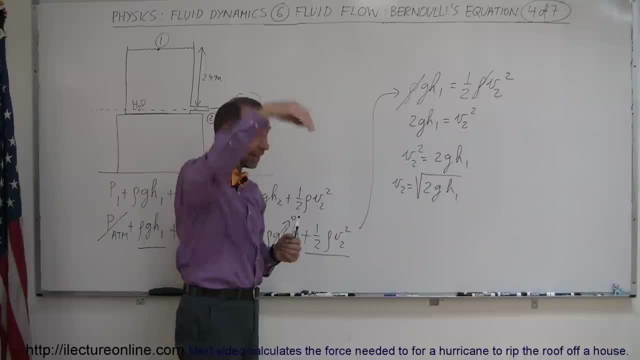 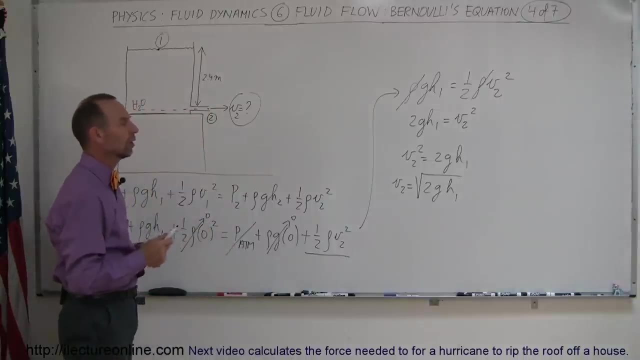 if you drop an object from any height, the velocity that it has when it gets to the bottom will always be equal to the square root of 2 gh1, if it doesn't lose any energy due to wind resistance or friction. So it's interesting how we get the exact same result using Bernoulli's equation to find the 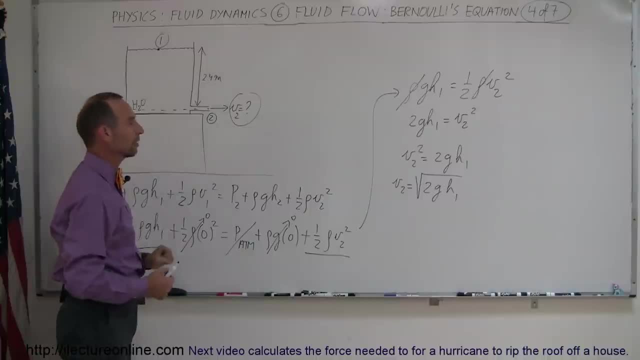 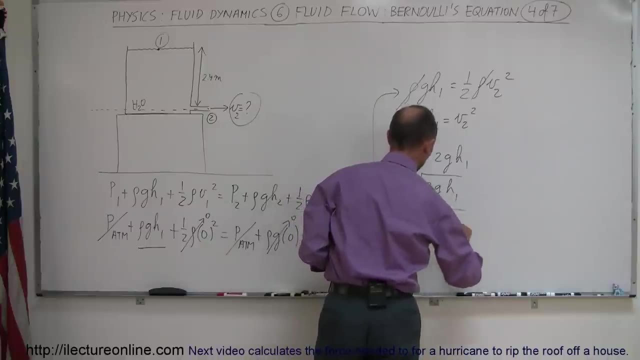 speed of the water as it emanates through a small opening from a water tank from that height. So let's now plug in the values. So this is equal to the square root of 2 times 9.8 meters per second squared times the height we said was 2.4 meters. Now we need a calculator. So 9.8 times 9.8 meters per second squared times the height we said was 2.4 meters. 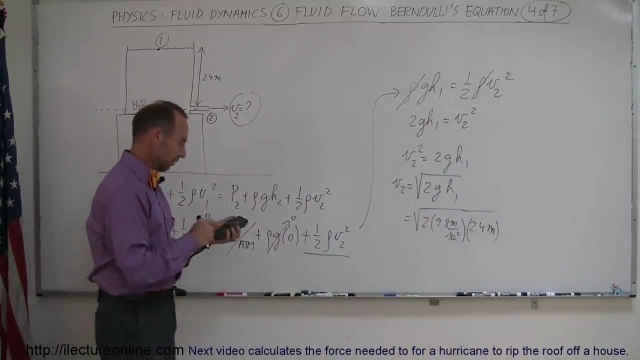 Now we need a calculator. So 9.8 times 9.8 meters per second, squared times the height we said was 2.4 meters. So now what you know where Herman has gotta prove the strength of the water tank has got. 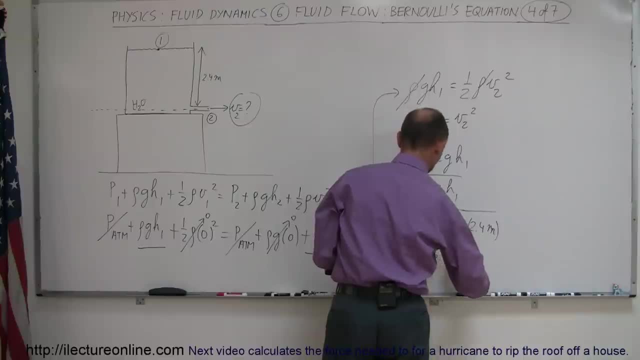 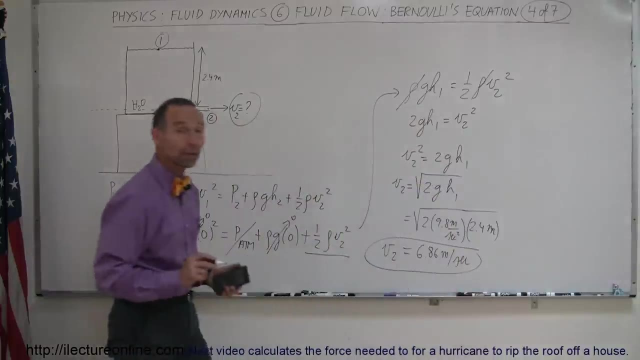 Here is what our Newton's plus and minus alumni's把它münf power of two times 2 times two point four equals and we take the square root of that and looks like it: 6.18. 6.енный from the block's exit to his water top. So we knew the sign Cortina 1 verbal equation to find the velocity of the water tank through that small opening at the bottom. and we need the plus and negociated one us that's high in ze nil de neon and we След trio 70 la neon per second e тер number 2 times 2 Per second for the velocity of the water läuft out of the water tank. 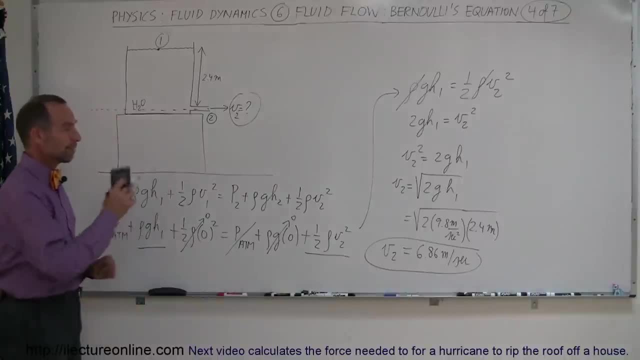 one- H2,, V2, solve for the unknown, and that's how you get the answer. All right, if that was a little confusing for you, we'll have some more examples to try and solidify the understanding of how to apply Bernoulli's equation in the next several examples.